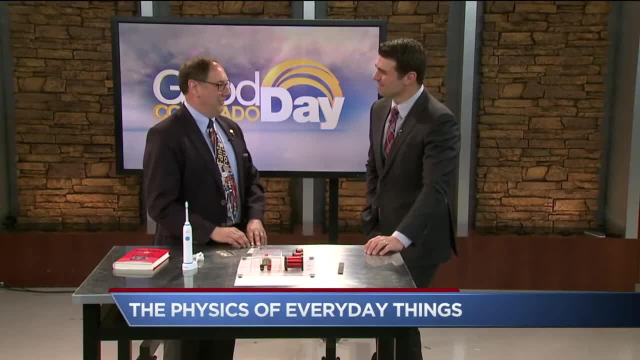 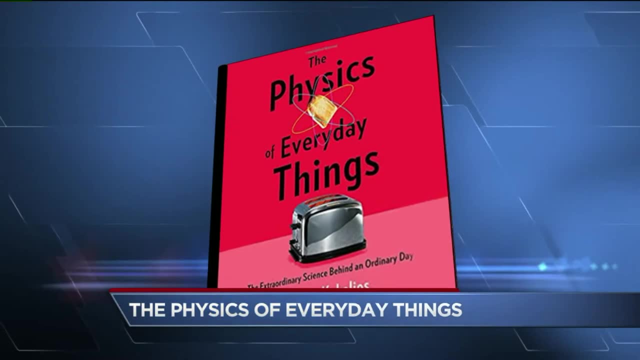 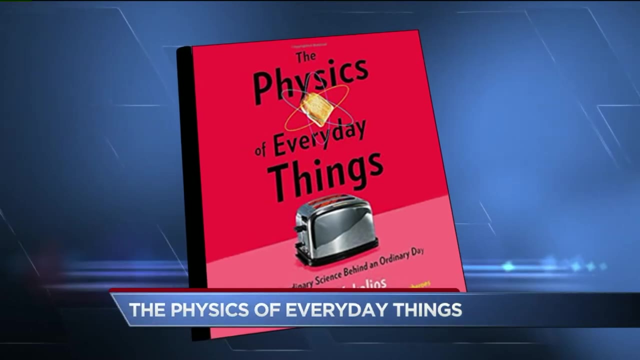 Kids, Kids, teenagers, grown-ups, senior citizens- everyone, It's for everyone. Once you see how the superheroes do it, you learn about the physics In the new book. you're the superhero and you go on the amazing adventure of an ordinary day, and I explain all the physics that surrounds you there. 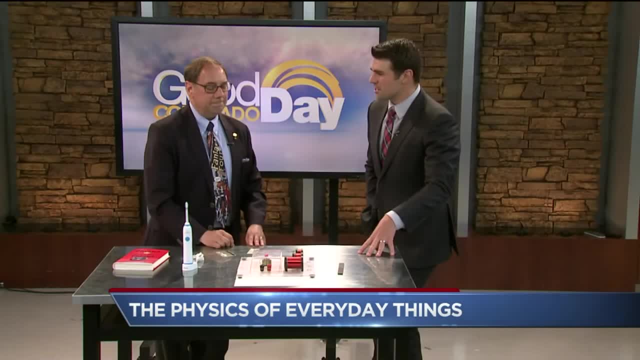 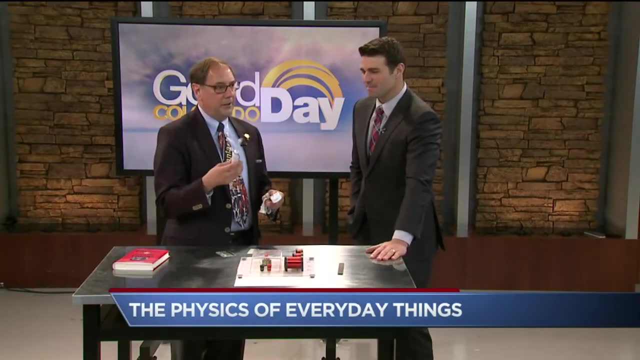 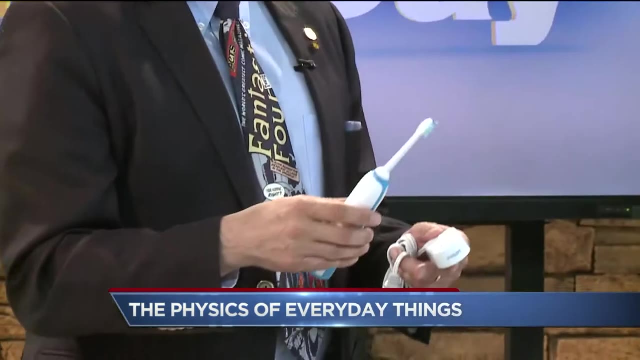 And there is physics in everyday's life, Modern marvels that surround us- your toothbrush, for example. So how does it work on that little charging base there? Sure, So there's a little motor in here And there's a battery power supply that gets the toothbrush bristles moving. You want to recharge it, but you have things that are going to be near water. 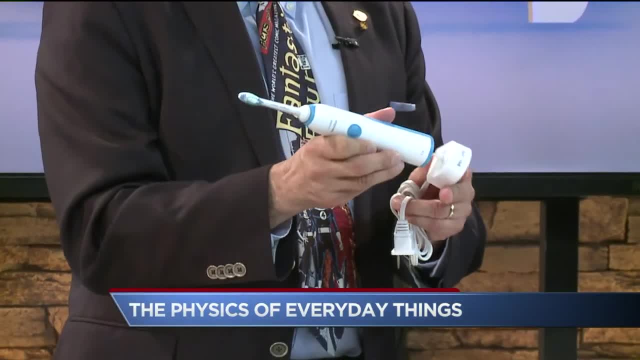 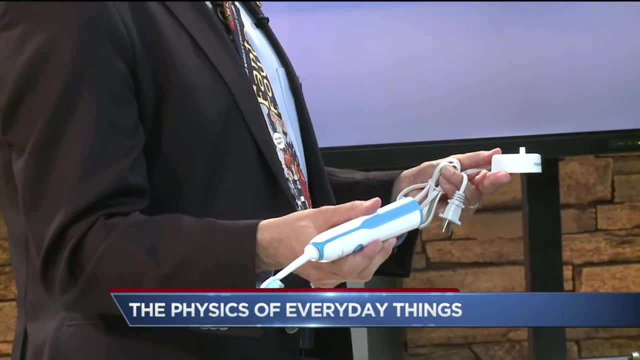 You want to plug it directly in, Correct. So you have a plastic charger here and you have a plastic base. Now, plastic and plastic are not good conductors of electricity. Yeah, wires aren't made out of plastic, Exactly right. So the technique they use is something called magnetic induction. 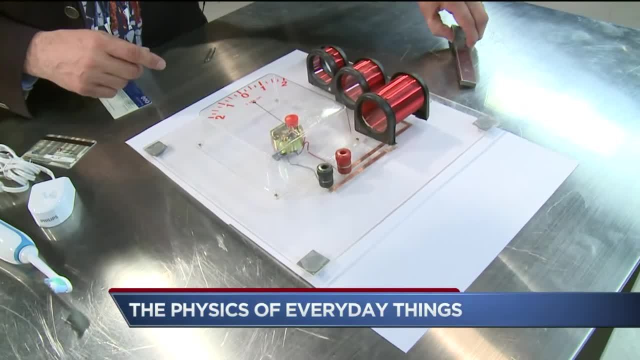 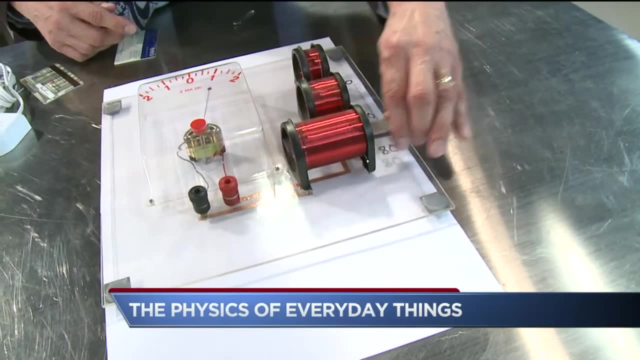 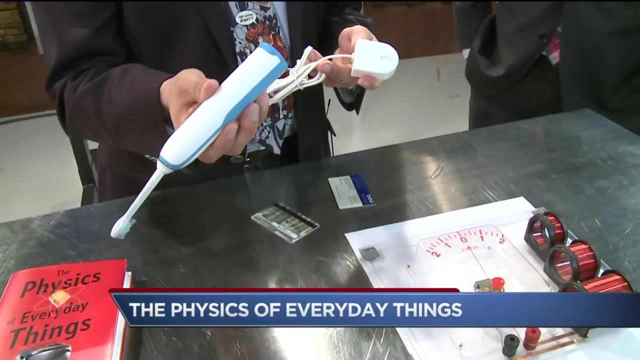 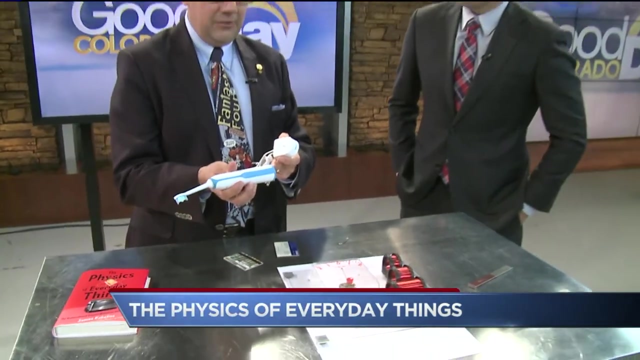 So we have a coil that's not connected to any battery and we see the meter is reading no current. But if I have a changing magnetic field I can get a changing current going through here. And so we have two coils: one in the base of the electric toothbrush charger and a coil in the base of the toothbrush. A changing current creates a changing magnetic field. that then changes the magnetic field through this coil in the base of the toothbrush and creates a current recharging the electric toothbrush. 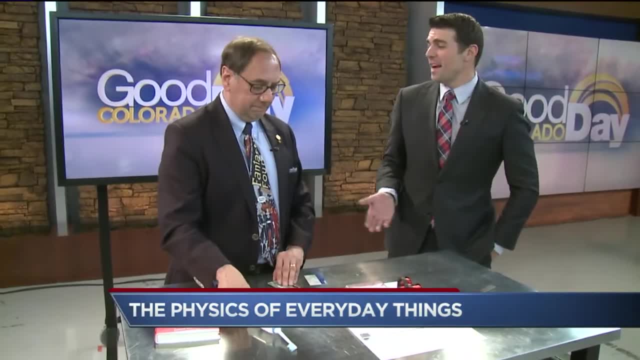 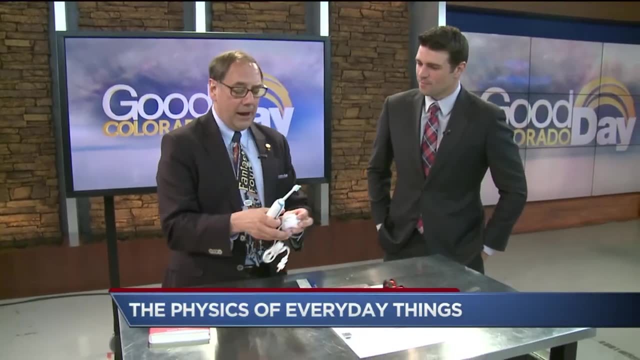 And the battery is connected to the battery, Done over an air and plastic gap, and you don't have to worry about any wires. That's right. These two devices or these two coils connected by a gap, is called a transformer. A simple device, but there's more than meets the eye. 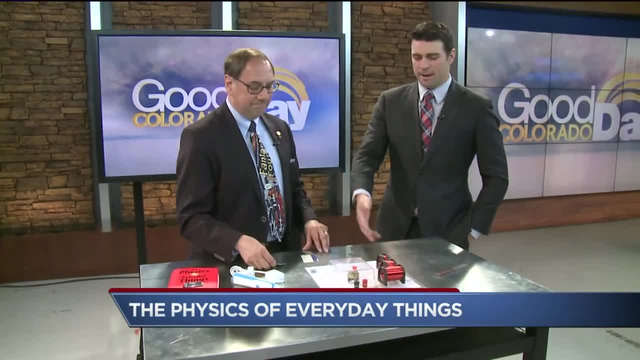 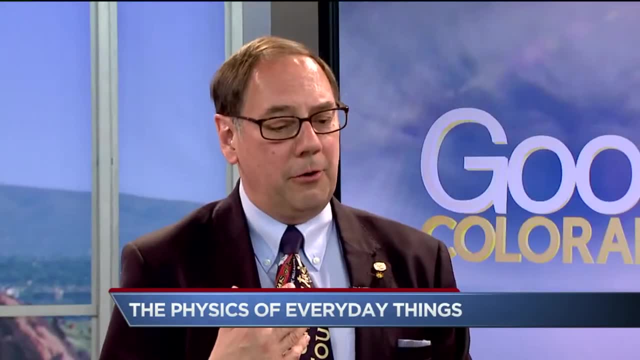 And it certainly is. And you know, you just stick your toothbrush on it and you're like: well, there you go, Magic, It charges up. That's all I worry about. sometimes, That's right, It seems like magic And as a physics professor, I thought it was very important to explain that it really is magic. 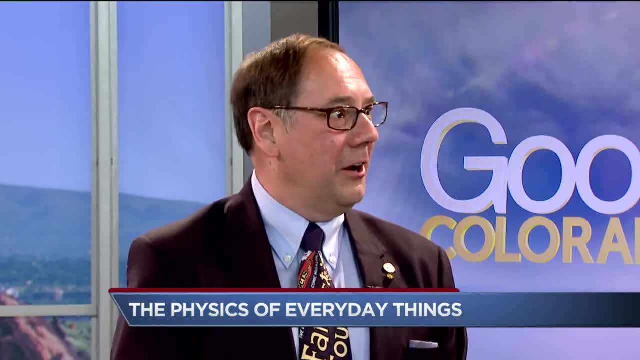 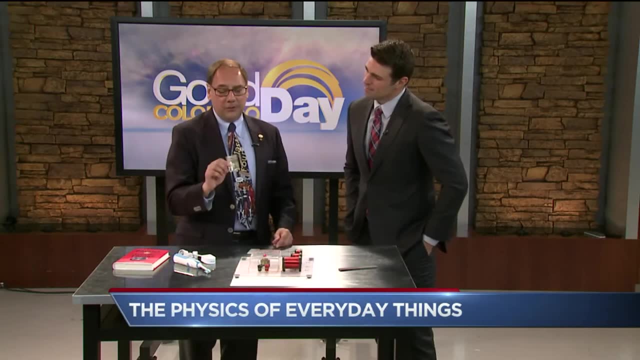 Yep, It's more like a Penn and Teller magic show, Right, Where they don't break the laws of physics but exploit them. There's more than meets the eye, Exactly, And so the same physics works on, say, your credit card strip. 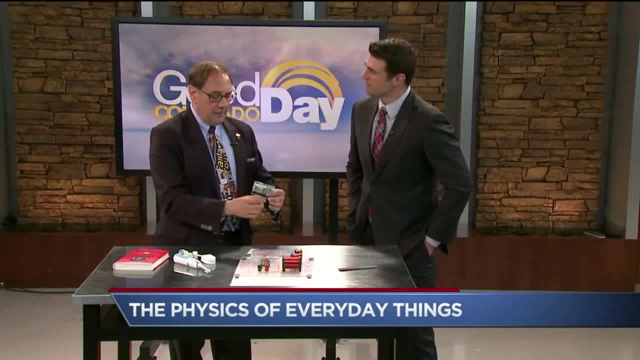 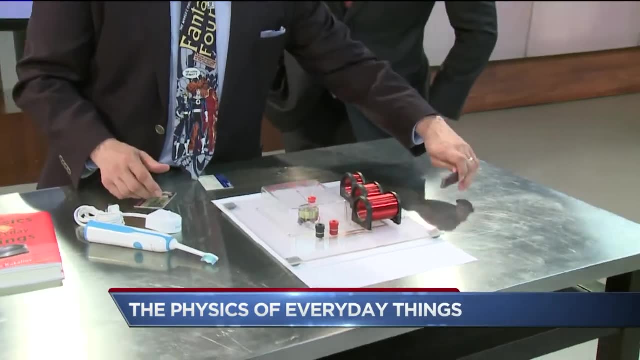 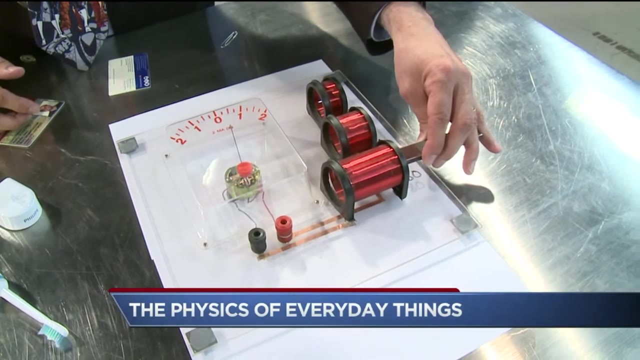 And when you pull the strip through the reader it scans the different magnetic fields and creates a voltage. And you notice here with the handheld that the faster I go, the larger the charge, And if I go very slowly I get a very small. 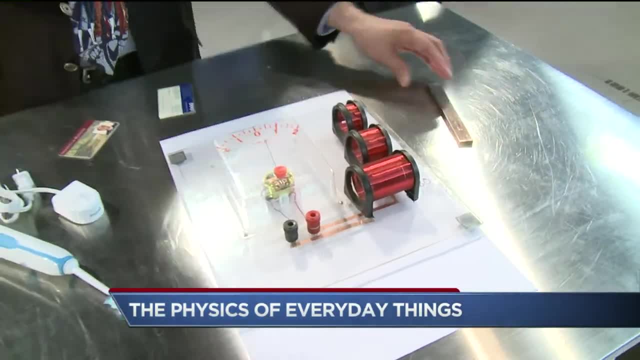 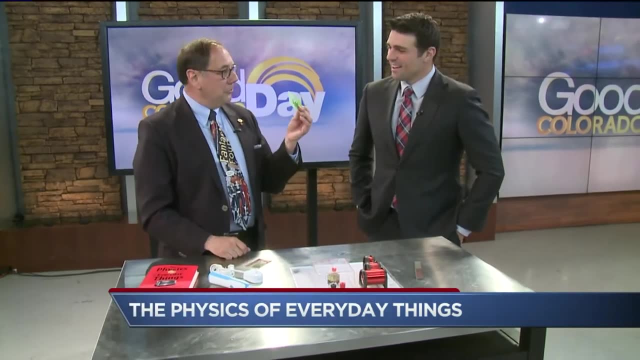 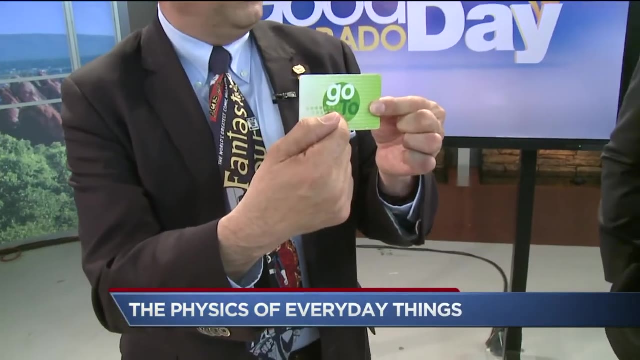 Small current And that's why sometimes when you pull the card it doesn't read And you have to go faster. You know, like again and all that kind of stuff. Your MetroCard has the same thing. There's a coil around the edge and a changing magnetic field, say in the bus reader or at your hotel. 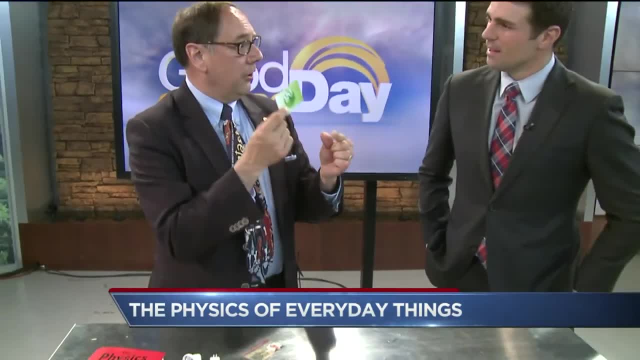 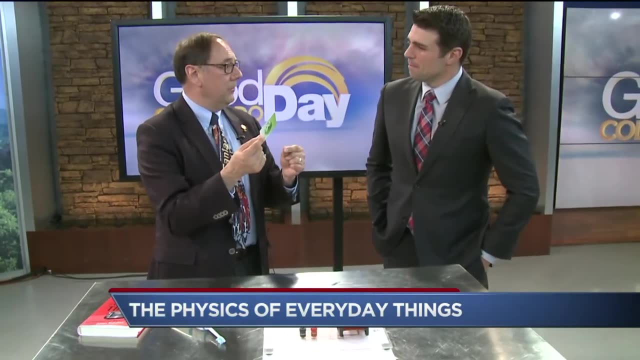 The changing magnetic field creates a current loop that charges up a chip that's inside here. that then sends information via the coil back to the reader saying how much it's going to charge, How much money is left on the card? or is this the identification code? 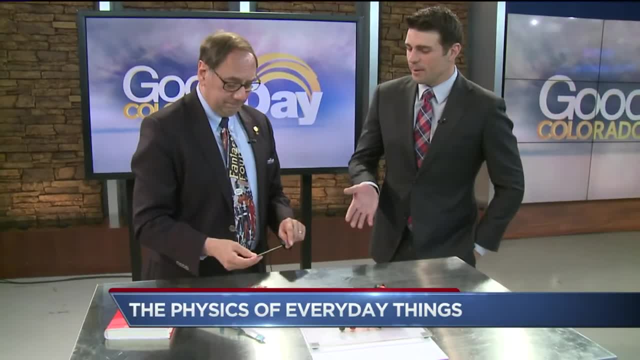 So this is indeed your hotel room And it's crazy, you know, to think that we carry all these in our wallets every day and you're just like, oh, here's the card up. The card works wonderful, but there's so much science behind it. 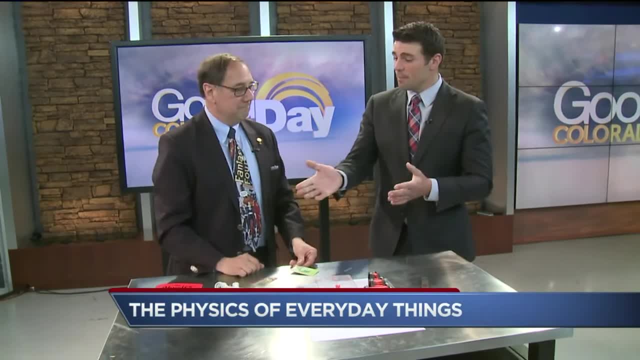 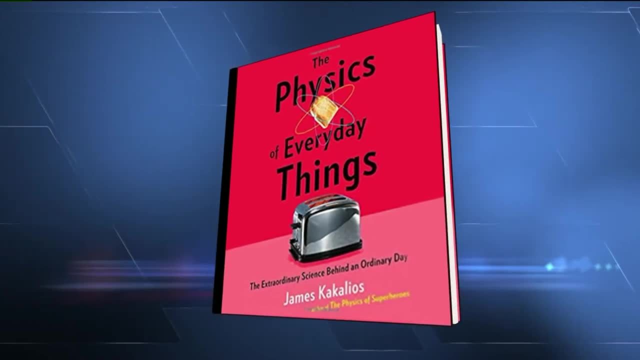 So much, And it's the same physics oftentimes. So you're going to be at a book signing tonight, right, Correct, In Boulder Bookstore at 730 pm. All right, And you can get the physics of everyday things. 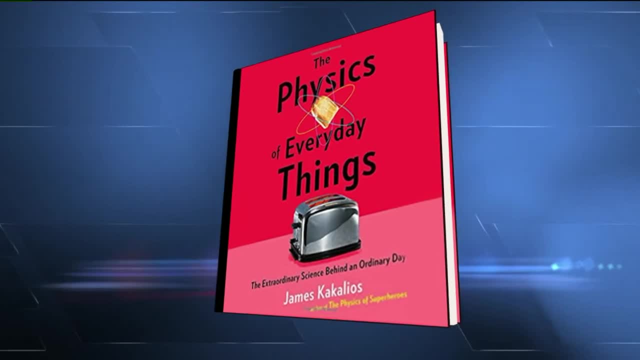 He's got other stuff aside from the toothbrush in there. Yes, it's a great. it's a great read for, You know, kids who may be interested in science or you want to get them interested. You can learn a few things from it. 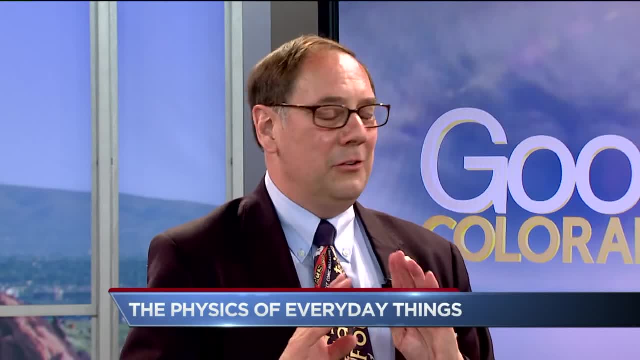 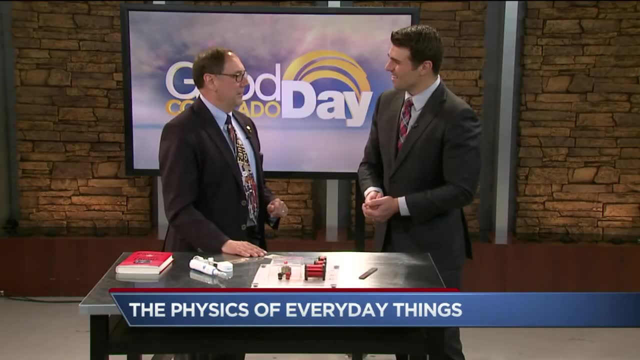 So, absolutely, We go everything from going through TSA to giving a business presentation, driving in using your GPS self-parking car. It's all explained there, All right. Well, thank you very much, James, Appreciate having you in. 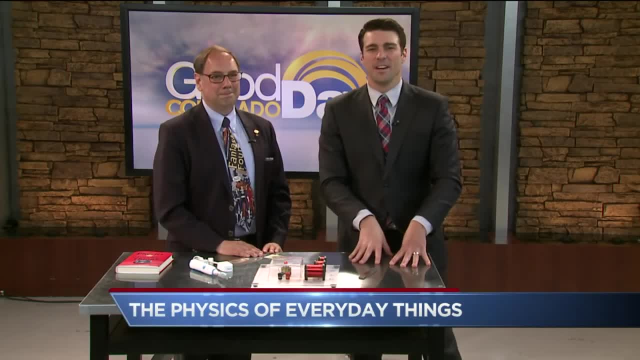 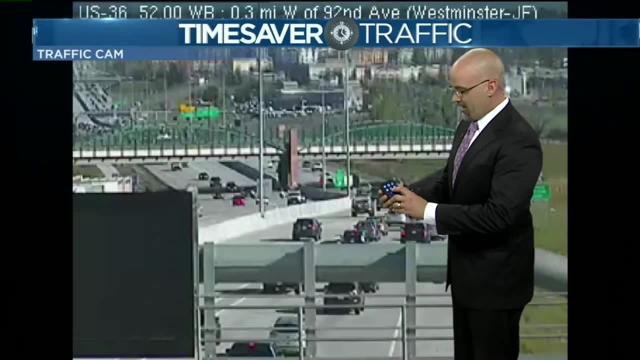 Hopefully some kids a little interested from the science behind the everyday stuff. Ken, can you explain the physics behind your little clicker there that does traffic? Yes, You hit this button right here. The power of the thumb That's, it Speeds along.